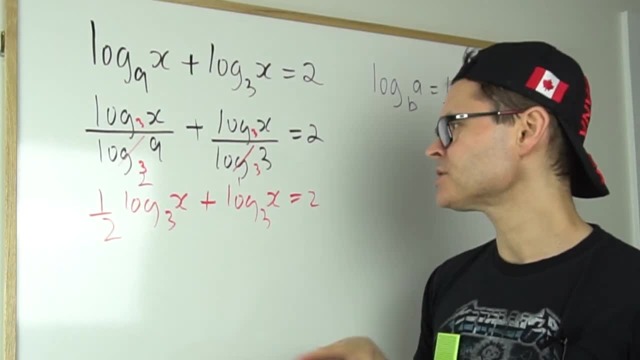 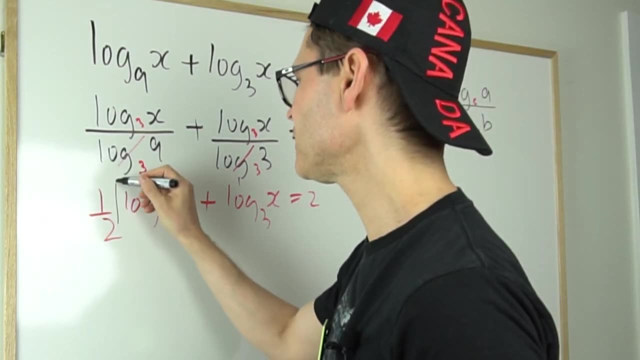 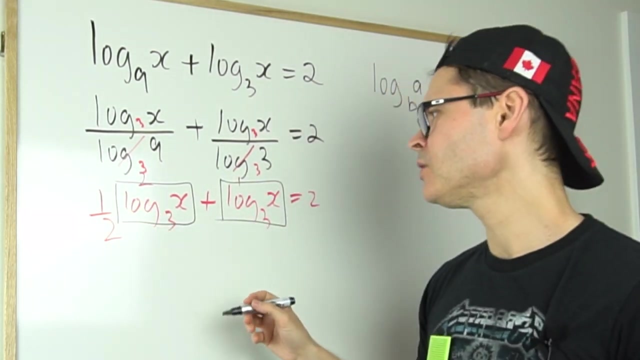 what i could do is i could, um, choose to multiply through by two, uh, but what i'm going to do is because these are like, for instance, just look at the log of x base three, the log of x base three. here i have a half of one, here i have one. so in total i've got three over two of them. 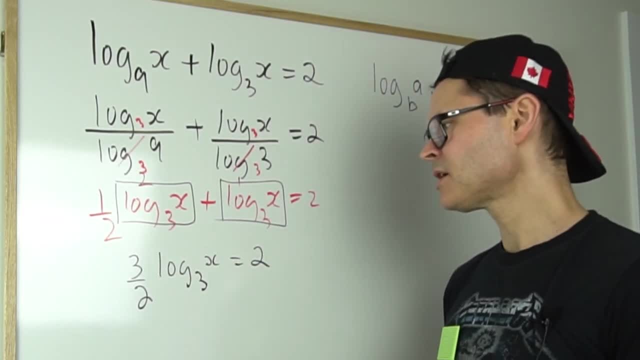 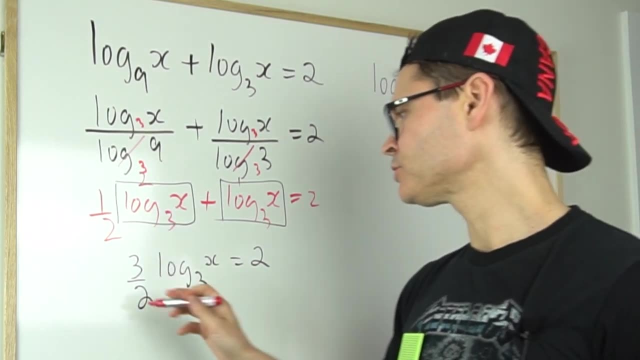 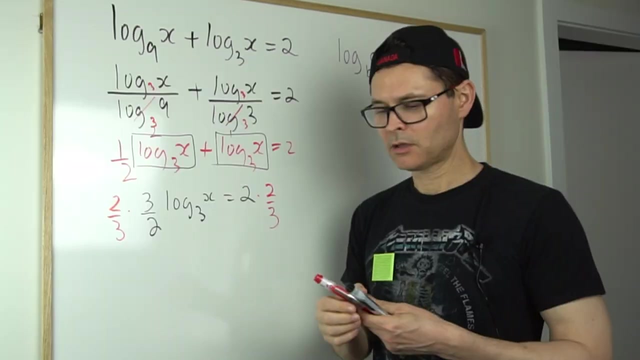 and you can see we're pretty close to cracking this, because what i could do now is, well, i could just multiply both sides by two over three. so if i multiply by two over three, by two over three, then it isolates the log, and now i'm in a position to be able to simply 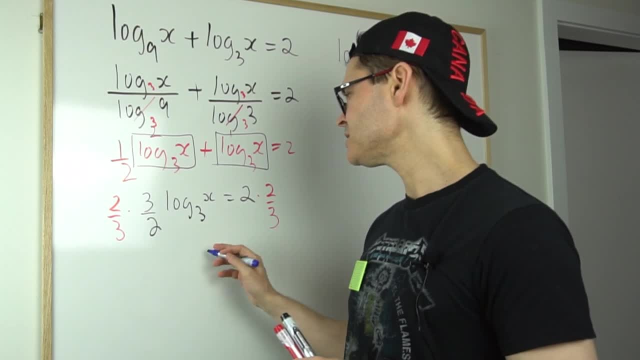 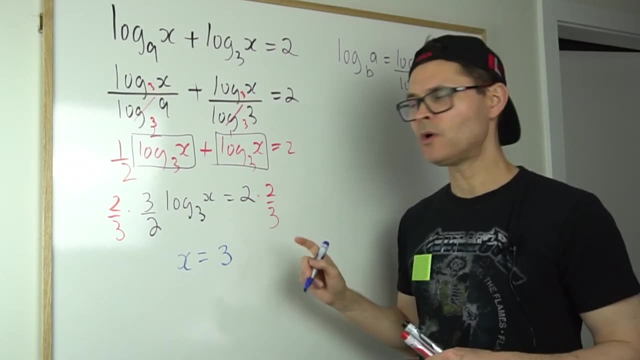 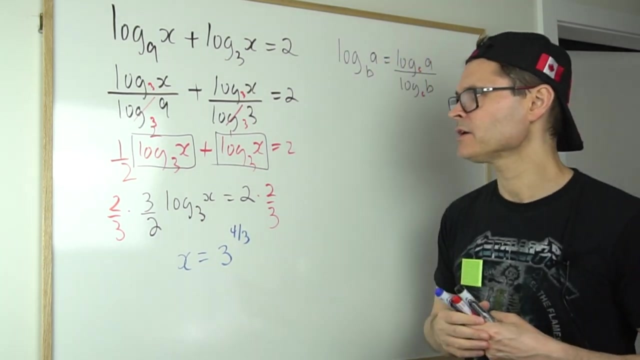 rewrite it from log form to exponential. so i could simply say now that x is equal to three. well, four times two over sorry, two times two over three is four over three to the four over three. i could have gone a different route here. if i had multiplied through by two, that would have given me 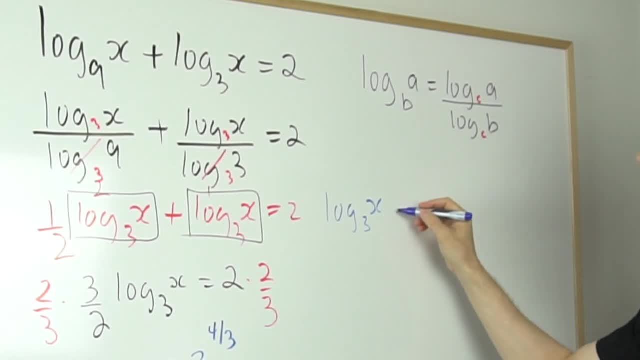 at this stage, the log of x base three over two over three over three, and so what i'm going to do now is i'm going to the log of x base 3 plus log of x base 3.. What I'm going to do? well, let me just erase this. 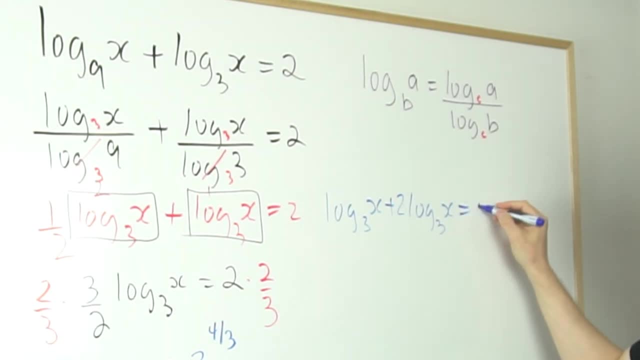 I'll put the 2 there. There should be a 2 in front of that Equals 4.. And then you could bring this up. Do you see? You could use your power rule And from there that would give me the log of x base. 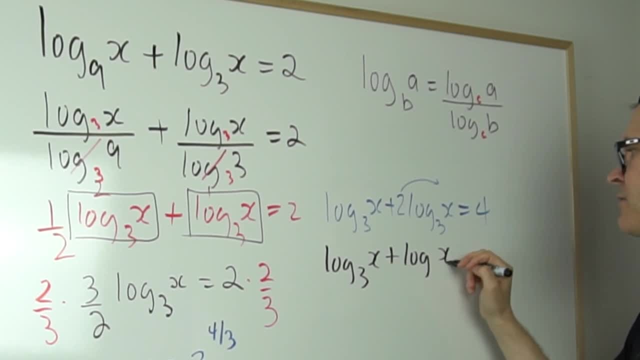 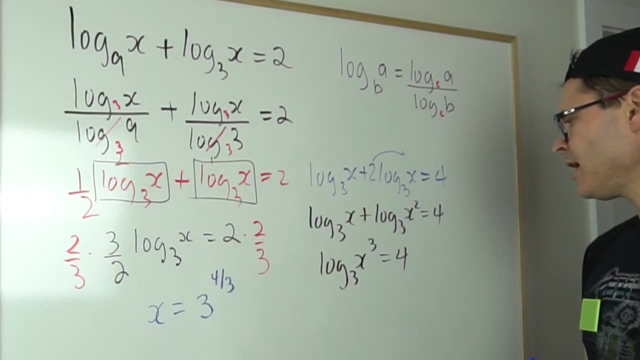 3 plus the log of x, squared base 3 equals 4.. And then I could use my product law by just combining that as a single log. That would be the log of x, cubed base 3, equals 4.. And then, of course here: 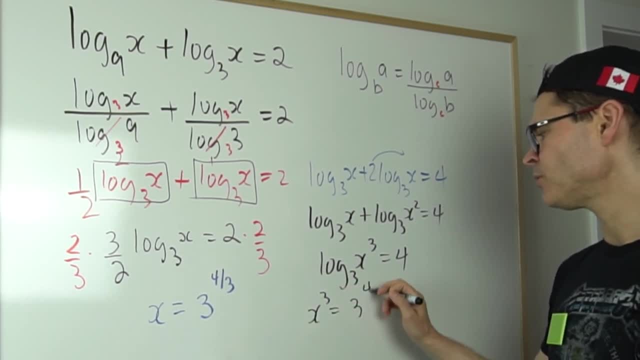 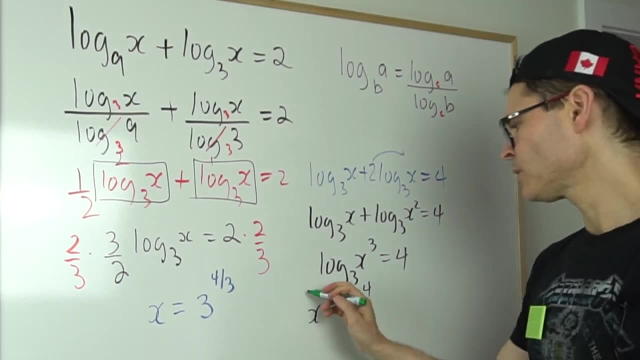 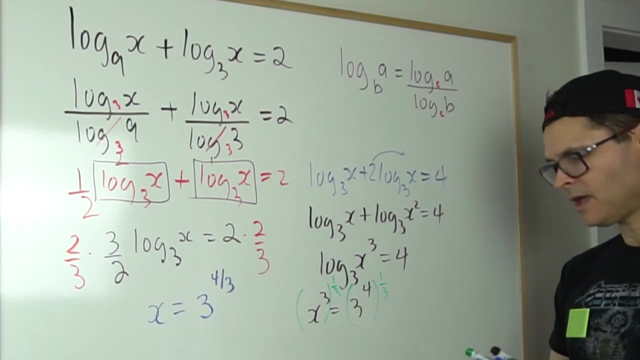 you've got x to the 3 equals 3 to the 4.. And I could simply raise both sides to the 1 over 3.. So raise both, Raise both sides to the 1 over 3.. 1 over 3.. 1 over 3. And I'm going to get the same answer. So the